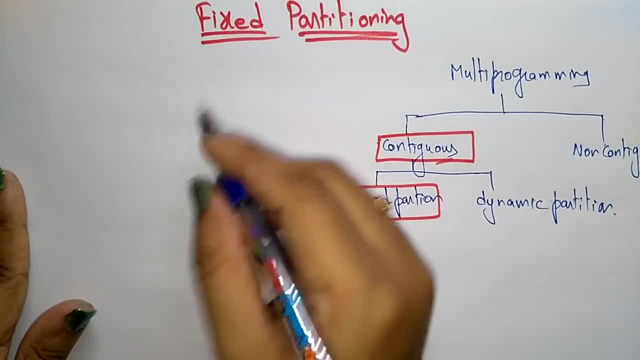 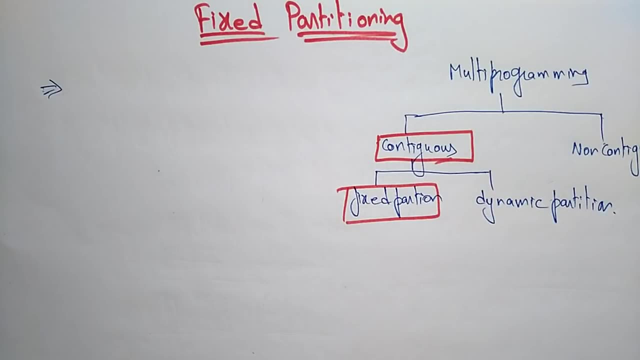 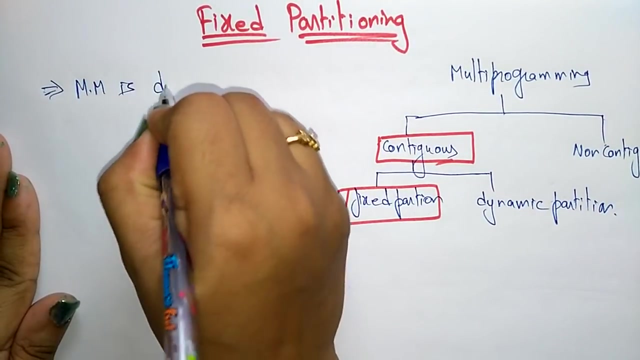 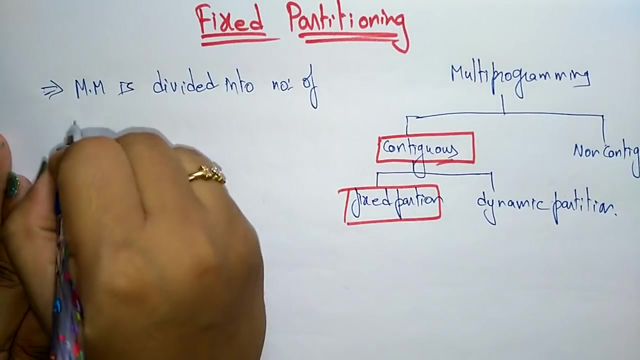 So what is this? fixed partition, A fixed partitioning here? everything, whatever the partitioning that we are doing by using the memory management techniques, that will be done in the main memory. The main memory is divided into. divided into number of static partitions. 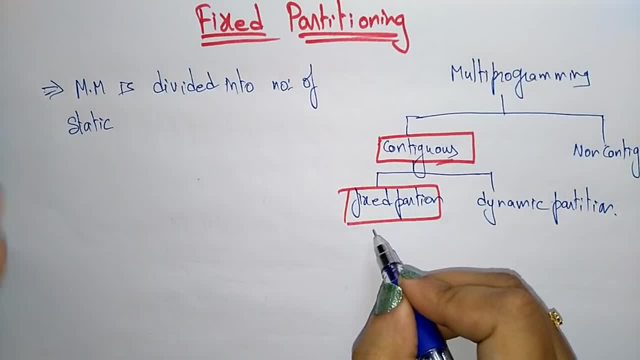 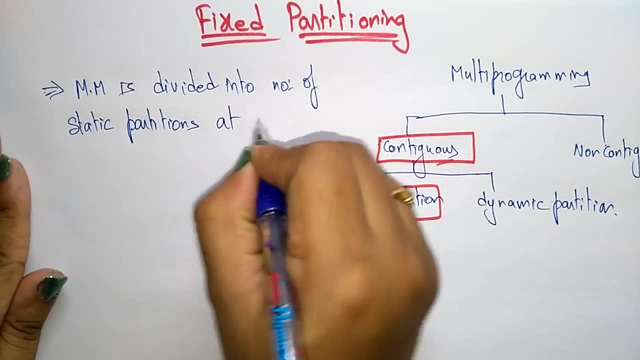 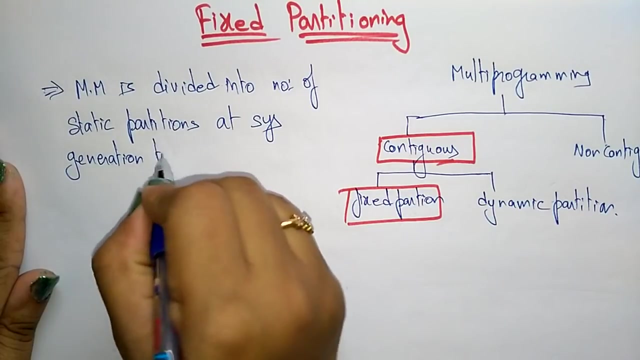 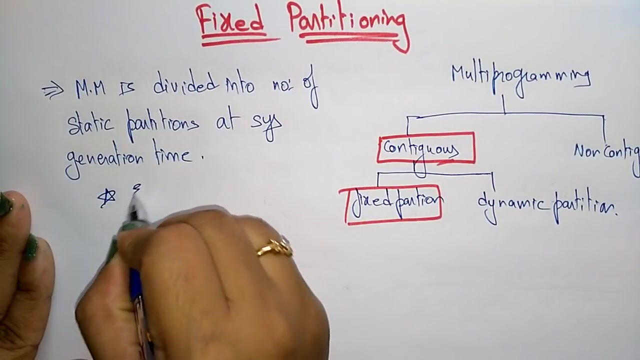 So we call it as a static. The fixed partition is also called as a static partition. Static partition is a fixed partitioning at system generation time. So this static partition or fixed partition may be, you can allocate in equal sized partition. 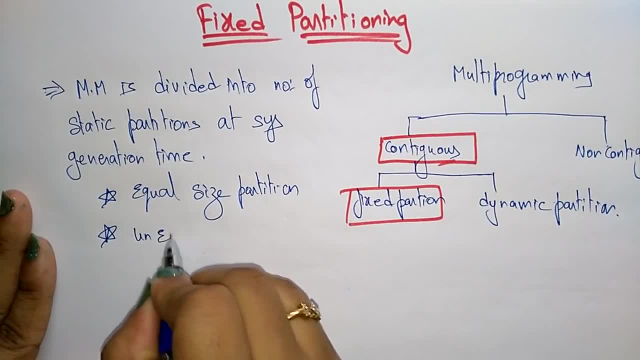 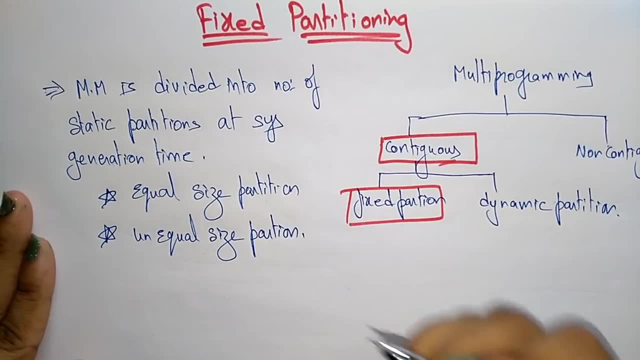 Equal sized partition or unequal sized partition. The static partition in the main memory can be done in the main memory location, be done equally or unequally. now let us see what are the pros and cons of this fixture partition. after that I'll take one example. the pros is it is simple to. 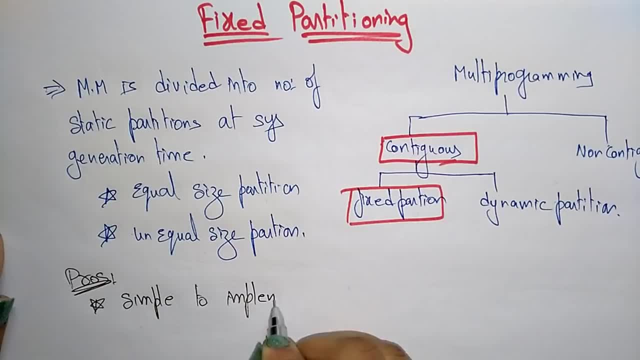 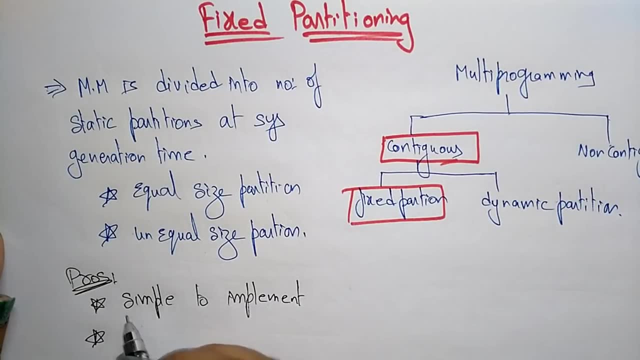 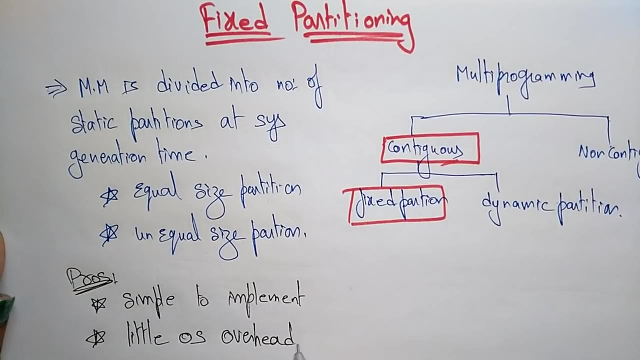 implement. the first advantage of using the fixture partition is simple to implement and here the only little or operating system overheads. are there little operating system overhead? why it's having only little operating system overhead? because it is a static partitions, so you are allocating the memory statically. it is a fixed partition, so that partition may be. 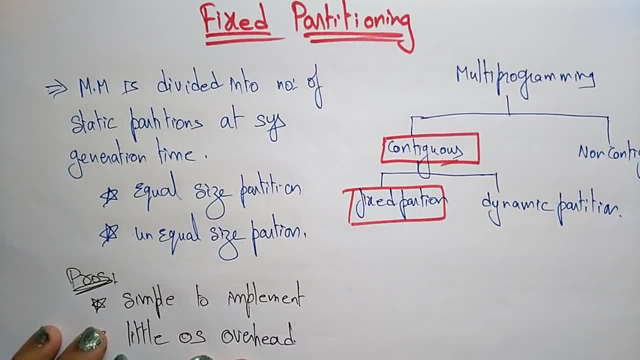 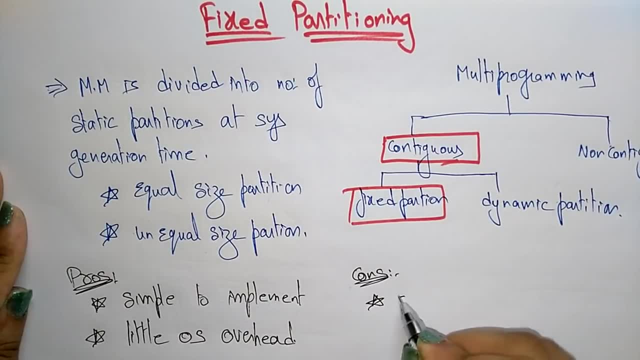 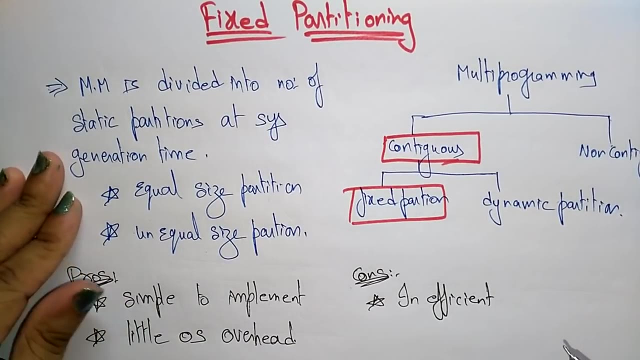 equal or unequal. so we are not using the dynamic here. so it is a little. OS overheads will be there and cons will be inefficient. so the first thing is this: fixture partitioning is inefficient, like internal fragmentation, so everything that occur in the fixture partition is inefficient, and here the maximum number of active process. okay. 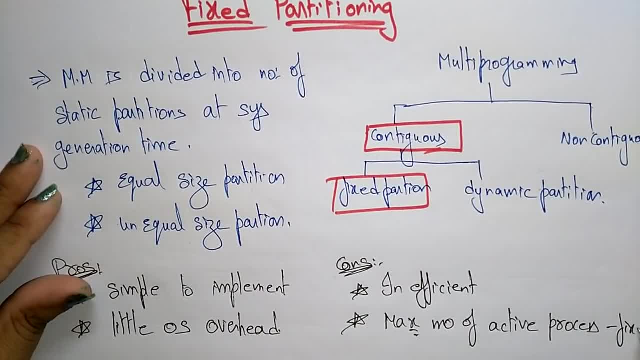 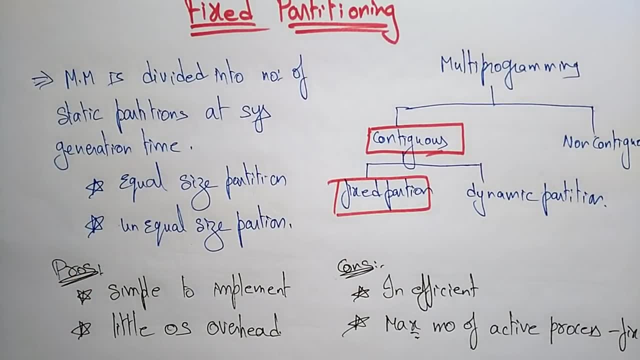 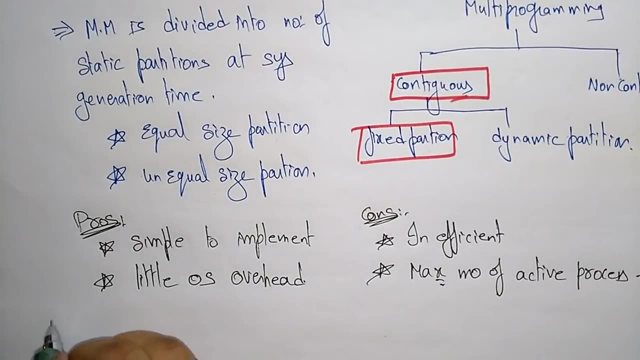 maximum number of active process will be present so that you call it as a fixed. so the party, the process that are allocating the memory that, or the fixed partition. so this is about the fixed version. now let us see what are the placement algorithm here we are using in fixture partition. placement algorithm means how 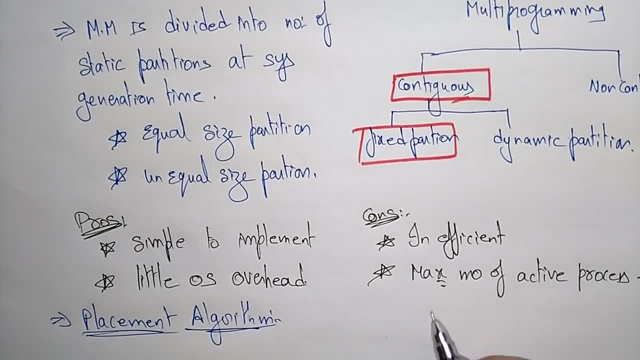 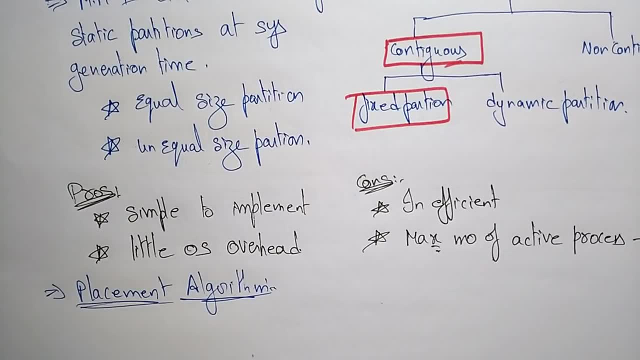 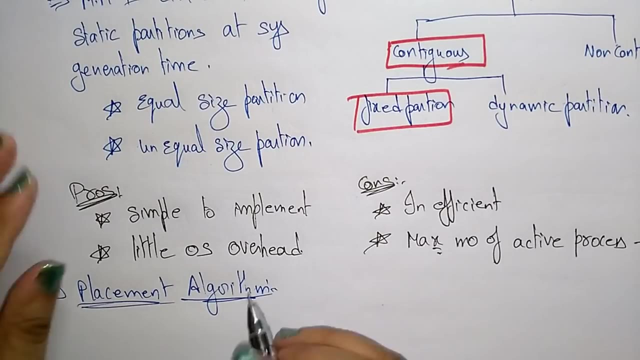 we are placing the process in the main memory. so you can use one process queue for partitioning per partition or you can use a single queue. so the placement algorithm for a fixed partition can be done in main memory by using one process, one process queue for partitioning, or you can go for a single. 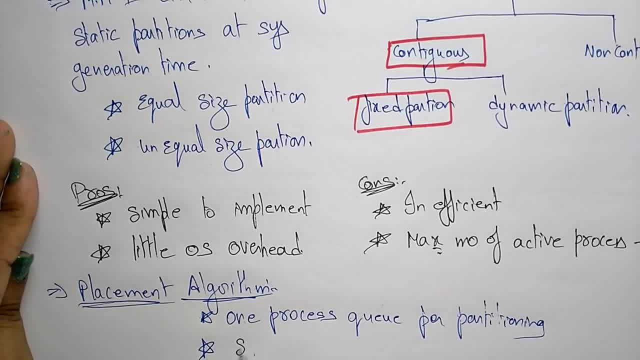 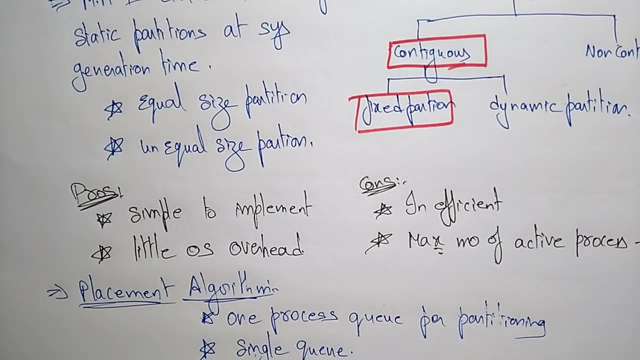 queue. instead of using the multiple queues, you can go for the single queue so the single part fixture partition can be done in main memory means we are placing the process that you call it as a placement algorithm. You are placing the process by using the Q per partitioning or single Q per partitioning. 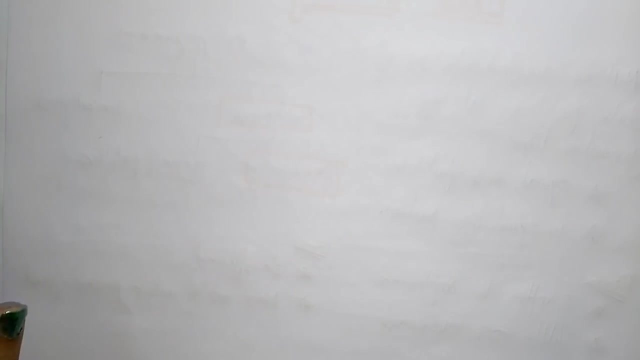 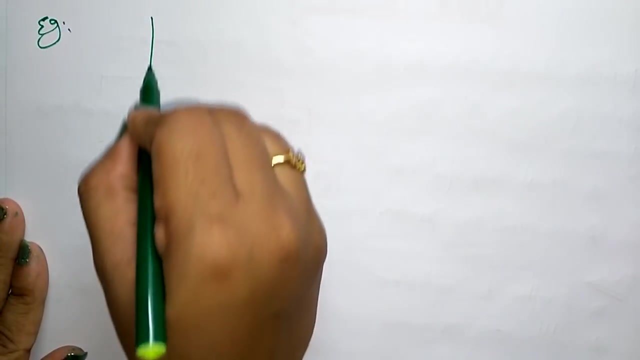 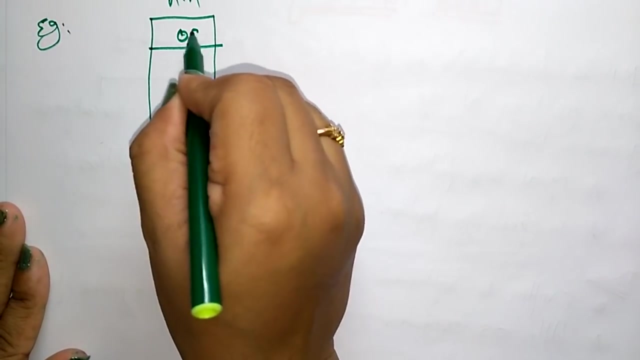 So let me draw this diagram: What is the single Q and the multiple Q example? So let us take: so this is a main memory, partitioning main memory. So first, here it is having the operating system, So the operating system is occupying the starting of the main memory. 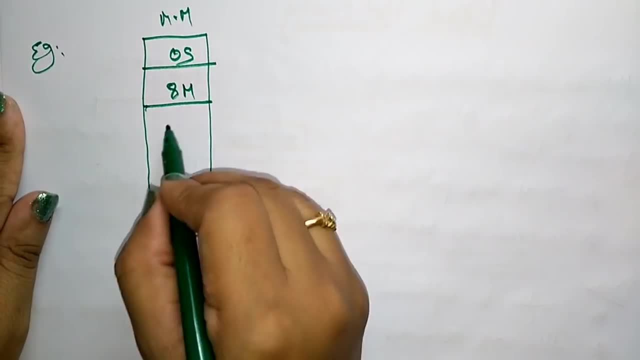 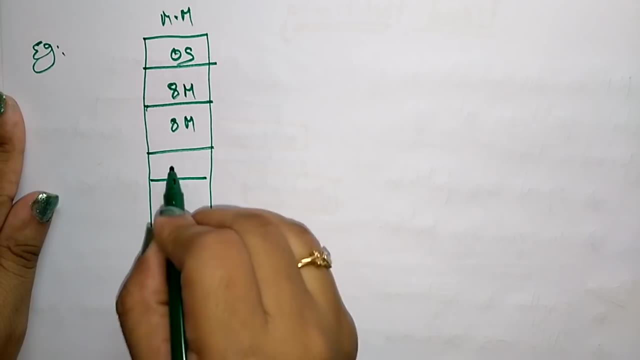 And here it is divided into. so I am talking about the fixed partitioning, So fixed equal size partitioning. First I am explaining about the equal size partitioning. So this you call it as equal size partitioning, Equal size partition. Now what about the unequal size partition? 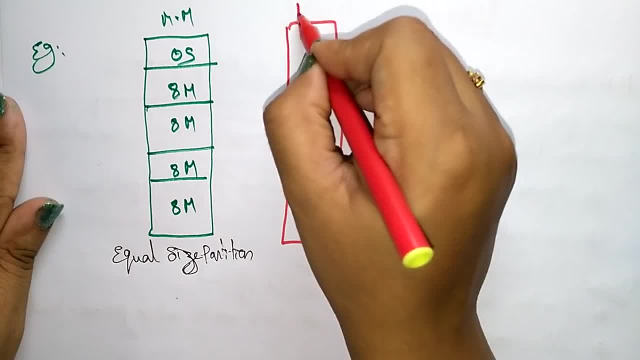 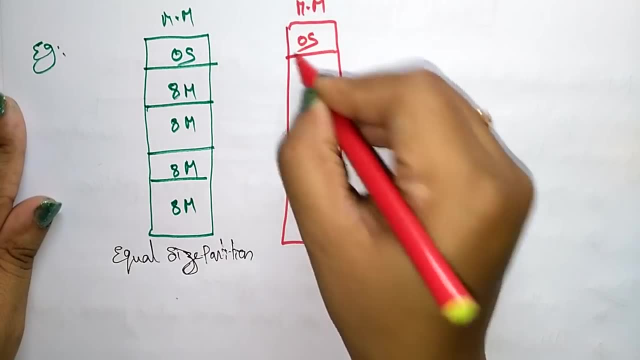 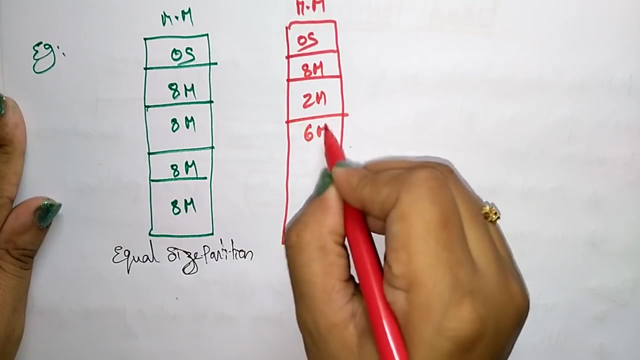 So the fixed partition can be done in two ways, In two types: fixed and unequal size. and unequal size. Unequal size means first the operating system, So you can allocate 8 megabytes, 2M, 6M, or you can go for again 8M, or you can go for 12M, like that. 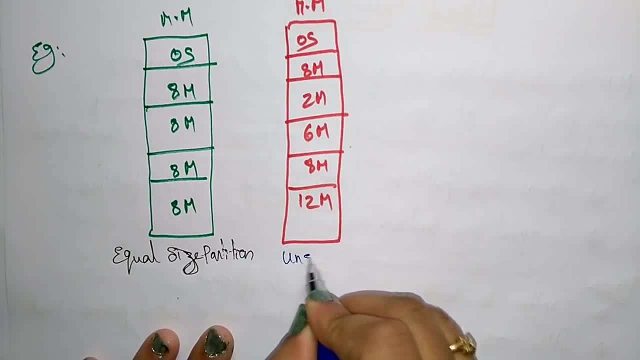 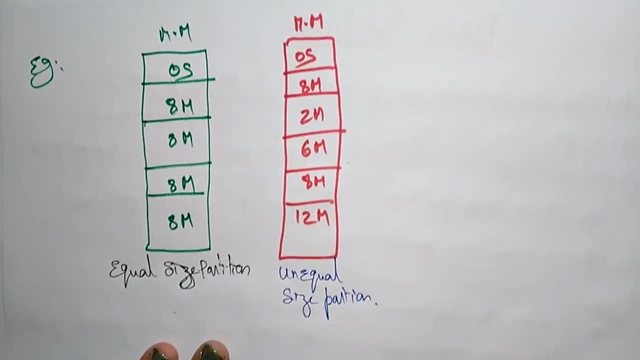 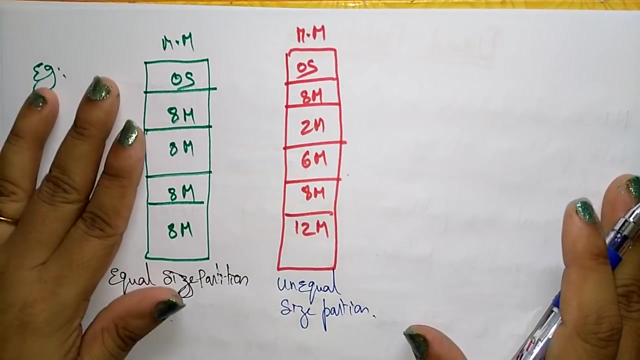 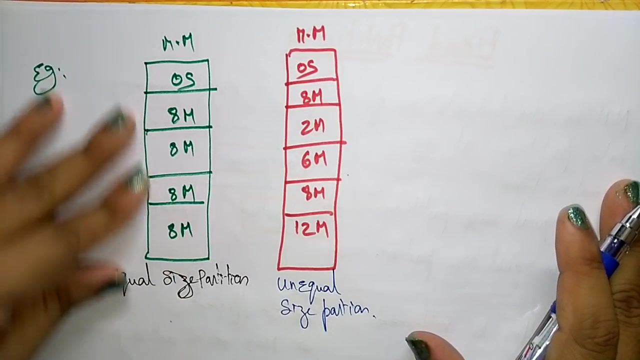 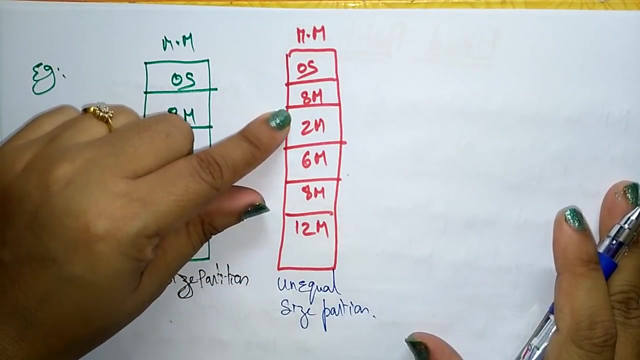 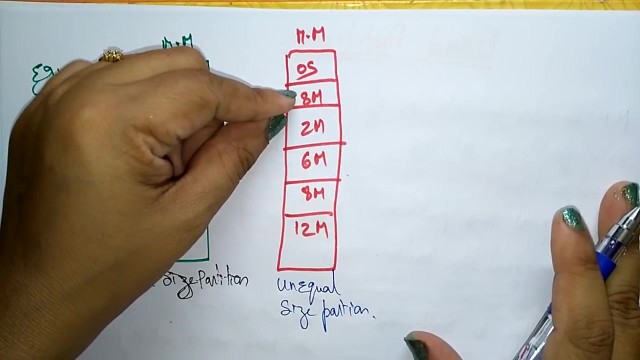 So this you call it as unequal size partition. Unequal size partition, So unequal, A fixed partition. so if you take 64 megabytes of memory, let us take, if you take the 64 megabytes of memory, the 64 megabytes of memory can be allocated like 8, 8, 8, so like that up to here. so equal size partition. unequal size partition means you can take the divide the memory slots into unequal sizes, but it is fixed, only the. it won't be changed. means one process can enter into only one slot, one chunk, one segment. 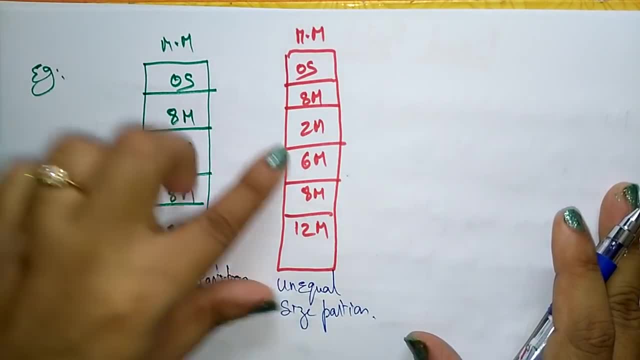 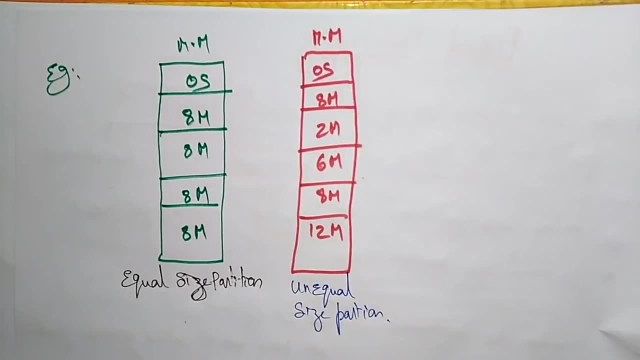 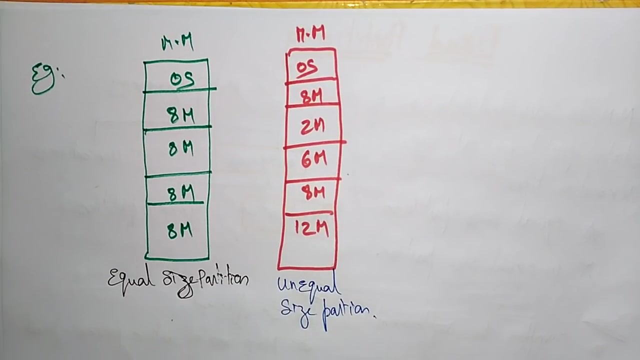 So 8M, 2M, 6M, 8M, 12M, like that. okay, this is unequal size fixed partition and equal size fixed partition. So let us let me explain about by using the placement algorithm. I said the fixed partition can be done by using one process, Q per partitioning, or single Q per partitioning. 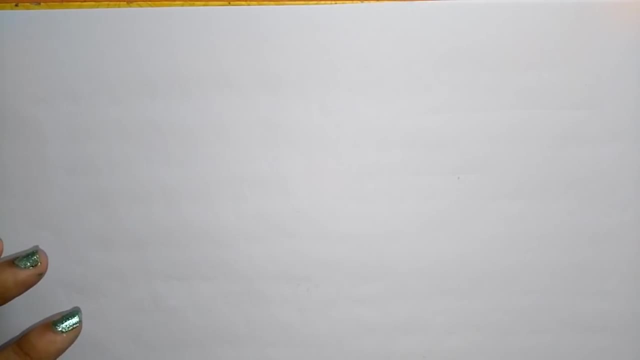 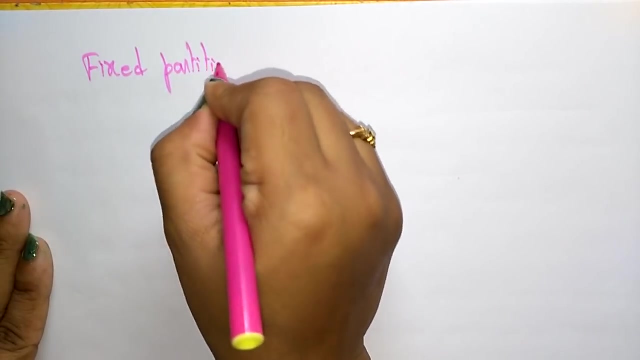 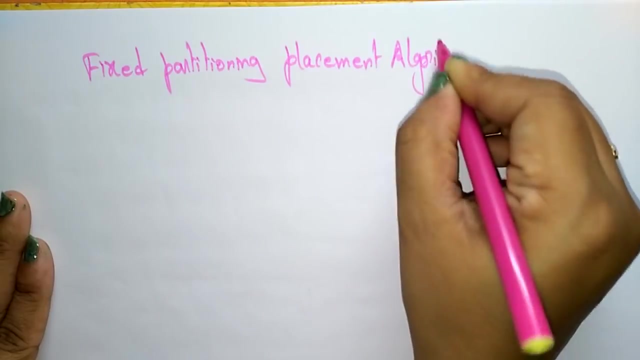 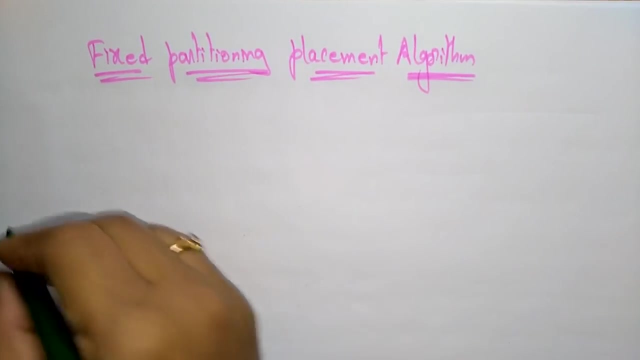 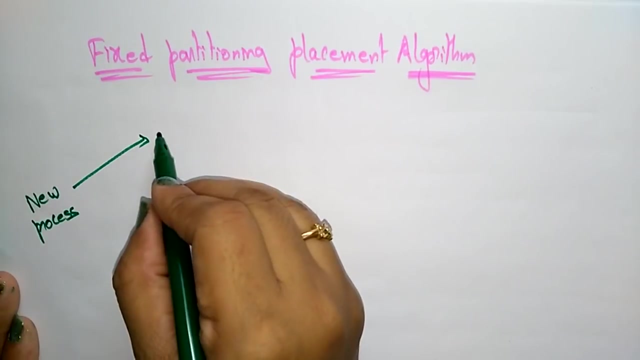 So let me explain that. So let us take Fixed Partitioning, Placement algorithm, Placement Algorithm. So here we are, taking suppose let us take a new process. A new process is divided into Multiple queues, means the data you're arranging in the queues. 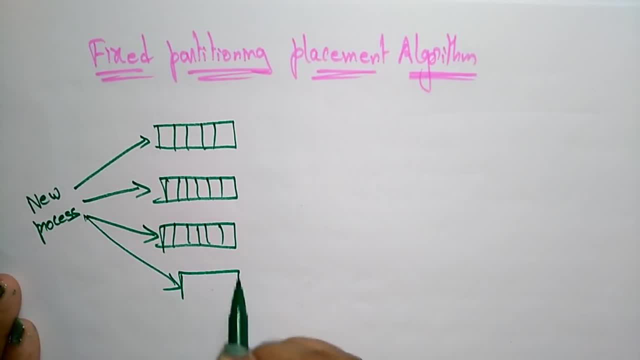 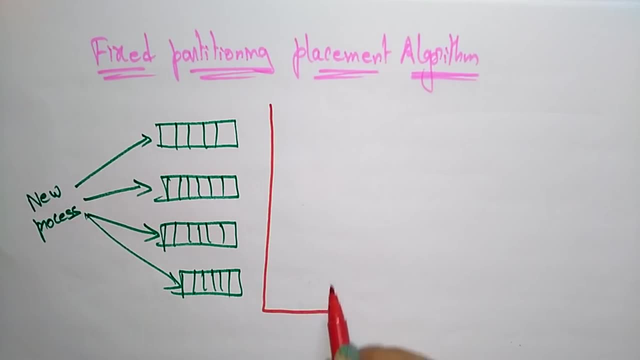 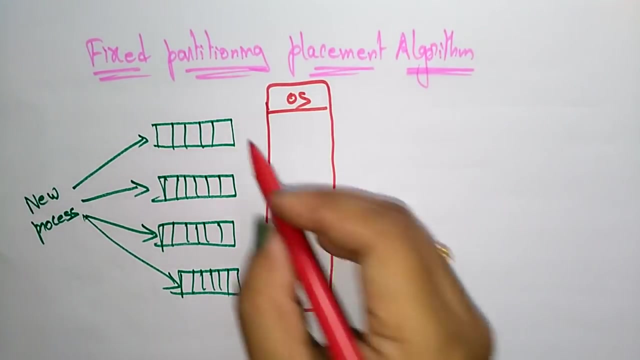 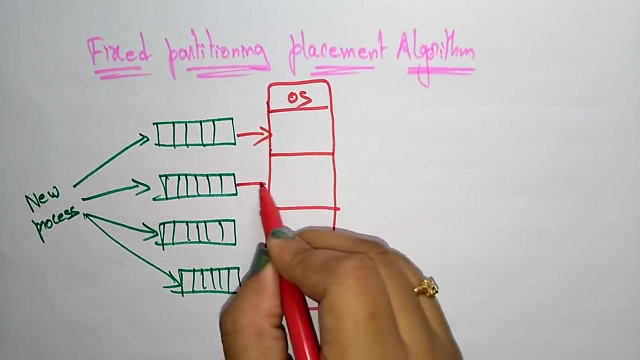 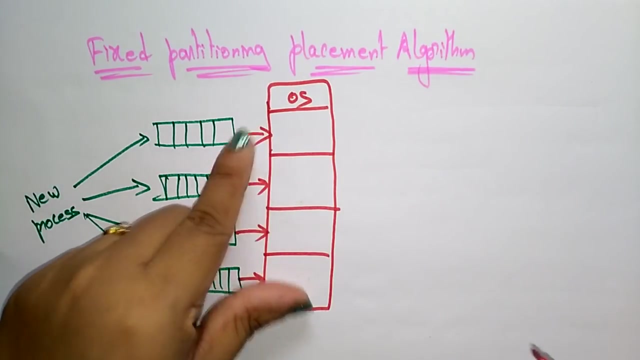 So like this, And here if you are taking the main memory, Okay, so this is a main memory. First, the operating system is stored and each queue will occupies One slot, one segment. So this you call it as one process, One process queue per partition. one process queue per partition. so for each partition, one process queue is arranging. 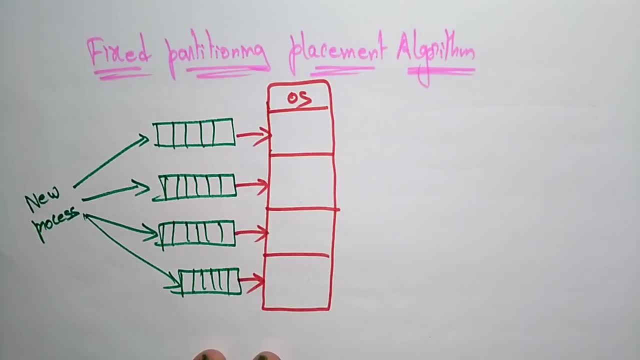 So if you take a single queue, let me draw that also new process, okay. so what I am saying here: in the new process you are taking only single queue. So this is a single queue. This single queue is occupying All the partitions.